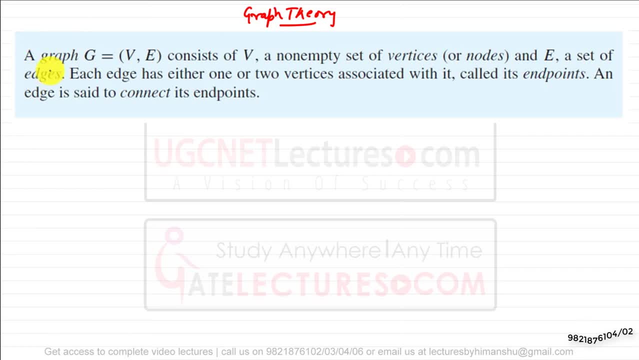 beginning, we understand what is the definition of a graph. so we can say a graph: G is equal to V, comma, E, see. graph is always represented in the form of sets, okay, where V is a set of vertices and E is a set of edges. so when I am 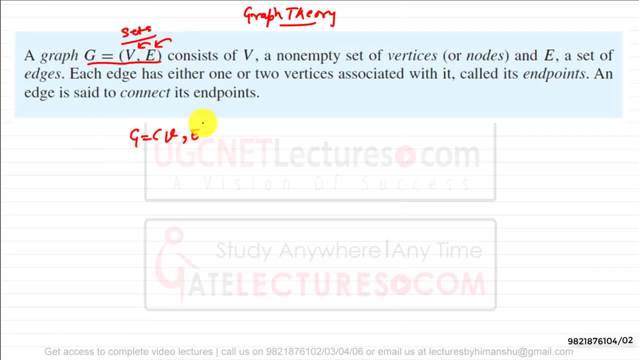 saying G is equal to V, comma E, where V is set of vertices and E represents the set of edges. okay, and these vertices are also called as nodes. now, each edge has either one or two vertices associated with it. I'm saying each edge has either one or two. 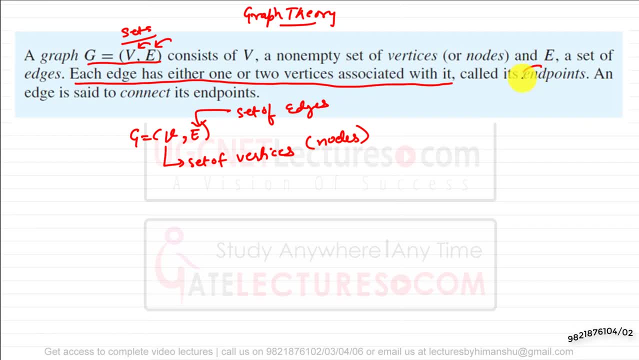 vertices associated with it which is called as a end-point of that vertex. for example, if I say: this is the first vertex V 1, this is the second vertex V 2 and this is a present in again H, even okay, so this H is associated with two. 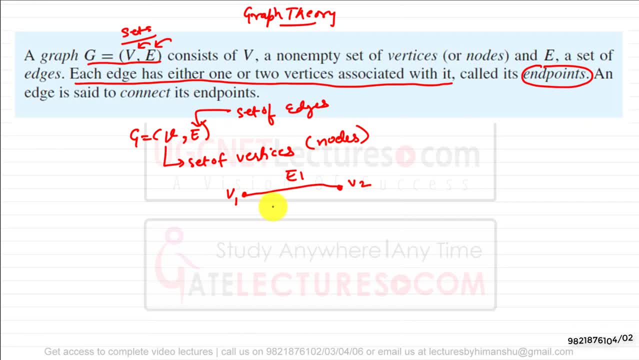 vertices, which is v1 and v2, which are also called as an end point of e1. okay, and an edge is set to connect its end points. now, this is how we represent a graph. now, for example, this is also representing a graph which is having three vertices: this is vertex v1, vertex v2 and vertex v3. this is edge. 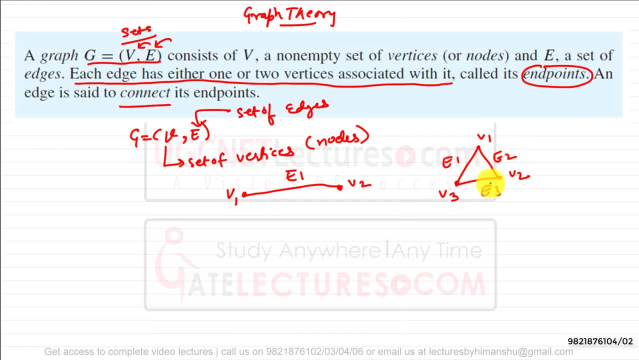 e1, edge e2 and this is edge e3. so what are the end points of edge e3, that is v3 and v2? what are the edge points of edge e2, that is v1 and v2? correct, now, there are different types of graphs. 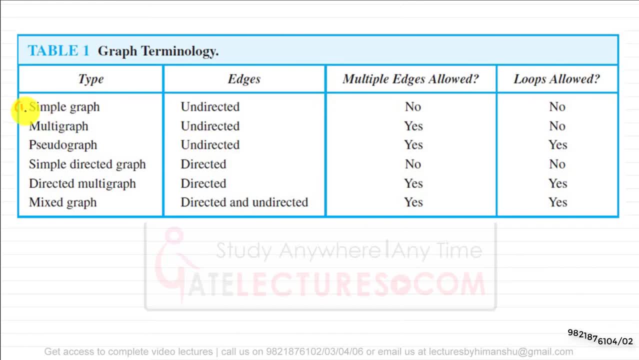 that are there. number one is simple graph, then we have multi graph, then we have pseudo graph, then we have simple directed graph, then we have directed multi graph and then we have mixed graph. now, what is the difference between these graphs? now, these graphs are differentiated within the form of: 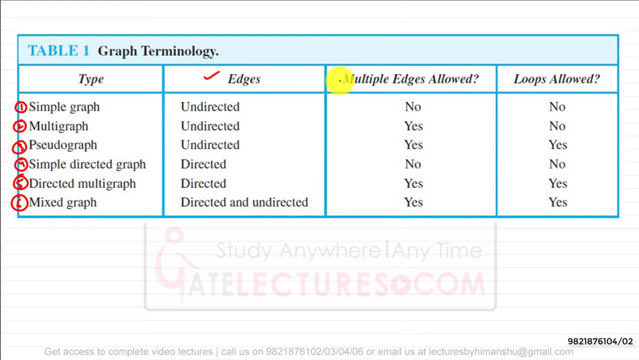 number of edges, the kind of edge they have, and do they have multiple edge or not, and do they have loops or not? okay, now, what is a multiple edge? multiple edge means between any two pair of vertices there are more than one edge present. now, for example, if i say this is a vertex v1, this is v2. 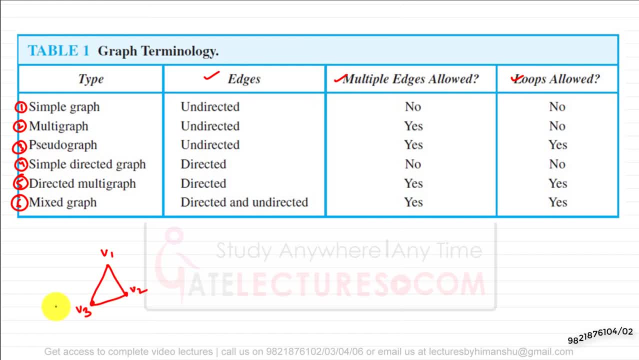 and this is v3. now, this is representing a simple graph, correct? why? because all the edges which are there, they are undirected. undirected, that means there are no directions given. so this is a simple graph. second, multiple edges are not allowed, like for example, between v1 and v2. there are no multiple edges. and third, one is: loops are not allowed. okay, 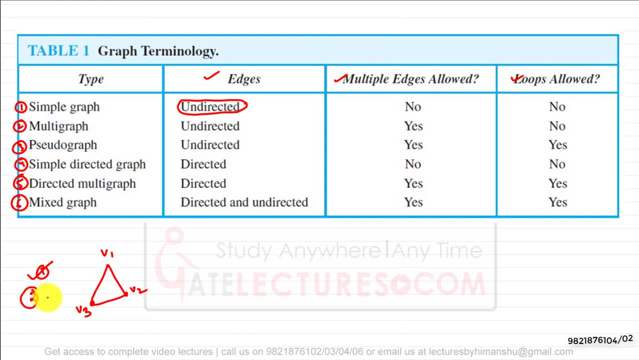 now, if i say: is this a multi graph? is this a multi graph? yes, it is also a multi graph. why? because it is undirected, even though we do not have any multiple edges, but still multiple edges are allowed and we do not have any loops. so this graph is representing a simple graph as well, it is also representing a multi graph. third, 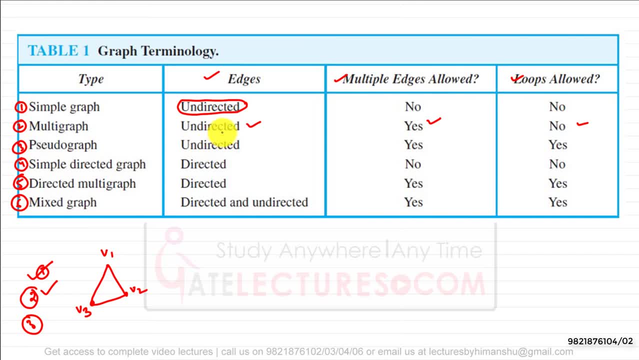 one is a pseudo graph. pseudo graph means it should have undirected edges. it can have multiple edges, but loops- sorry. it can have multiple edges as well as it can also have loops, so this is also representing a pseudo graph, correct? so this is just like we are giving more. 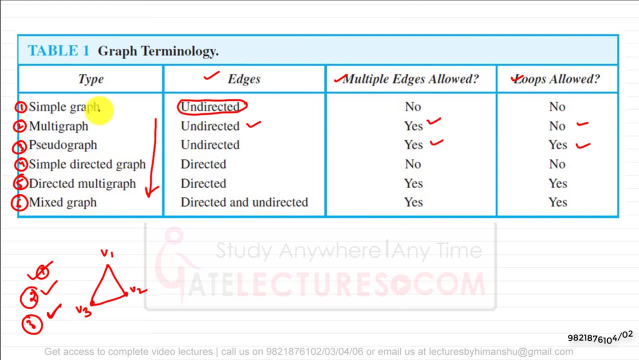 freedom in. in all these cases it means any graph which is a simple graph, it is also a multi graph, it is also a pseudo graph. now, if i say i have this kind of graph, this kind of graph, that is, this is the vertex v1, this is vertex v2, this is vertex v3. but in this graph we have two edges between the. 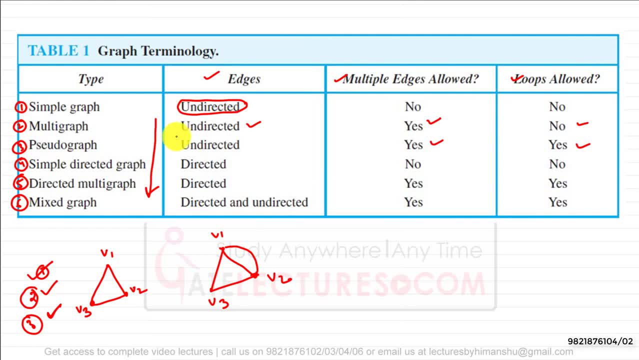 vertex v2 and v1. so these edges, if i say we have two edges now, for example, this is one edge, even, and this is representing the second edge, e2, so because there are two edges. so now this is not a simple graph. it is not a simple graph why? because 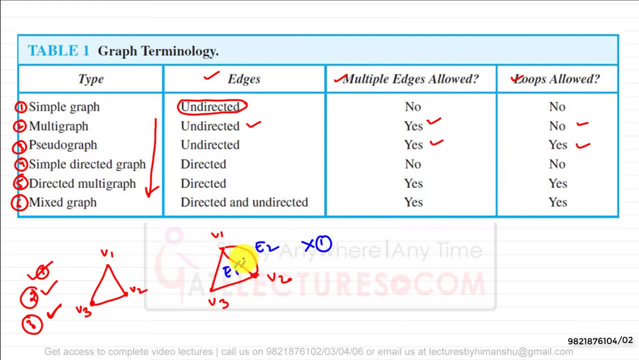 there are multiple edges between the vertex v1 and v2. these two edges are connecting the same pair of vertices. second, is it a multi graph? yes, it is a multi graph. why? because there are multiple edges, correct? is it a pseudo graph? yes, it is a pseudo graph, in the same way you 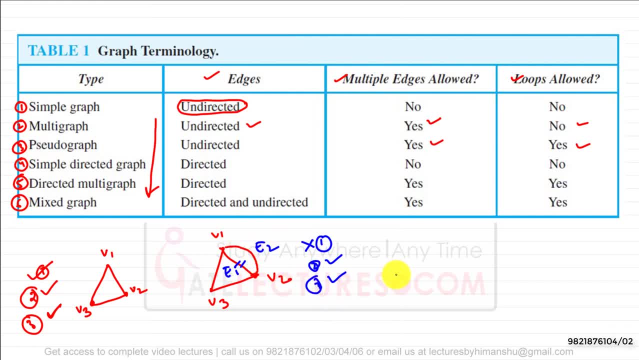 can find out for the other points also. now if i say: what is the pseudo graph itself? if i draw a graph like this: this is the vertex v1, this is vertex v2, this is vertex v3 and we have a self loop at vertex v2. okay, what is the self loop loop is where, uh, with for an edge, if starting. 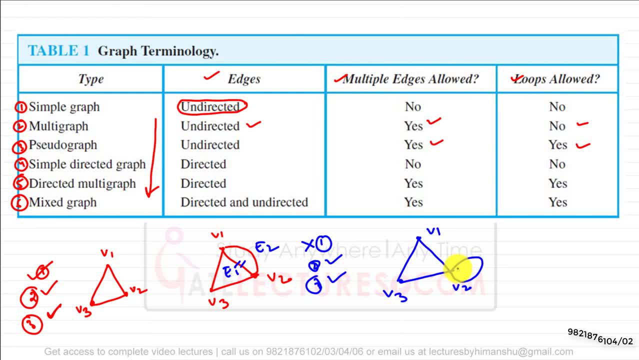 vertex and ending vertex. both are same. now that is called as a loop. now, is it a simple graph? no, why it is not a simple graph? because, uh, yeah, so because, for example, in between v1 and v2 there are multiple edges that are present. why, uh, it is not a multi graph? why, because, uh, in multi graph loops, 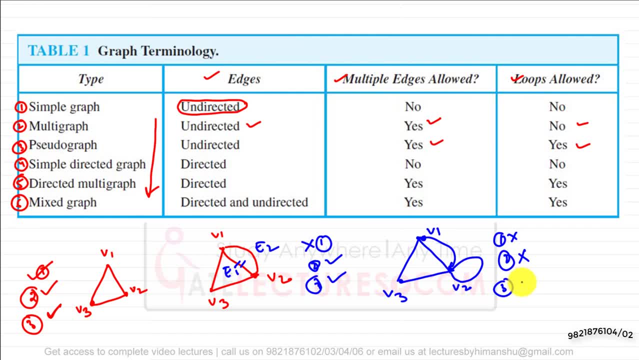 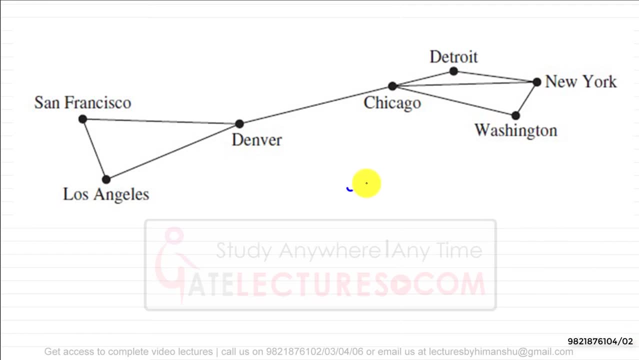 are not allowed, but this graph is having loops. is it a pseudo graph, correct? it is a pseudo graph. now we'll see just some examples of all these six graphs in the next slide. just have a look at this now. this is representing a simple graph. okay, as i told you what is the definition of a simple graph. 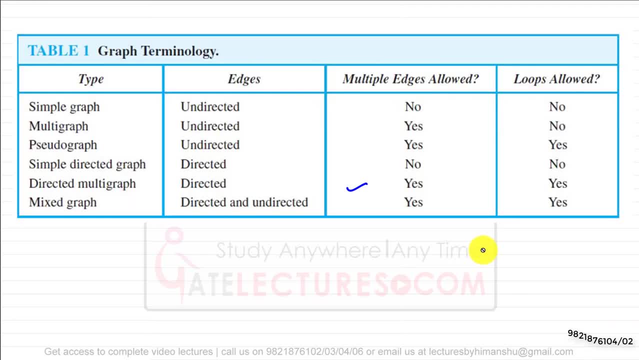 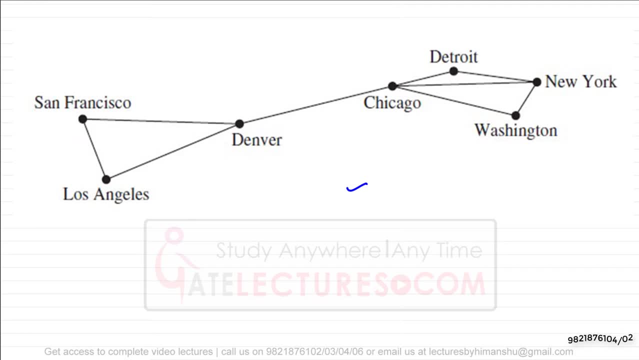 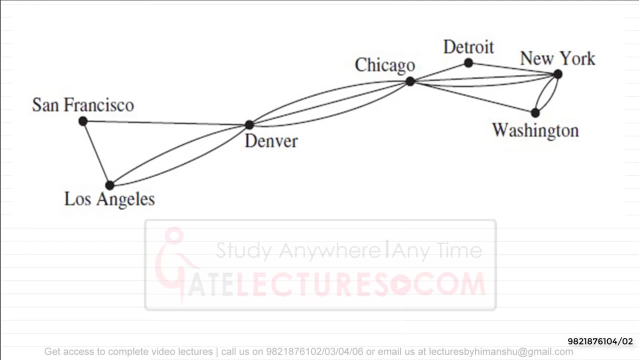 a simple graph is not having any multiple edges, and it is not all. it is also not having any kinds of loops, okay, so therefore, it is representing a simple graph. now, if i say this graph, now, this graph is not a simple graph, but it is a multi graph. why? because, in this case, 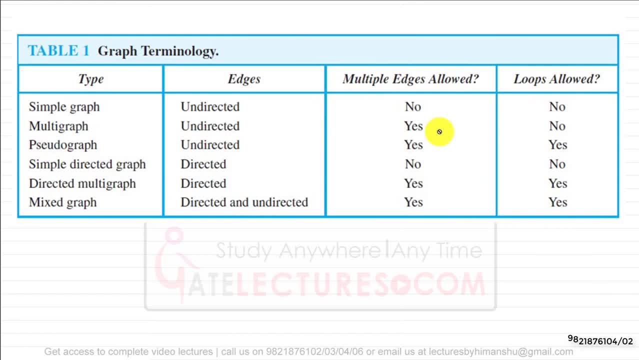 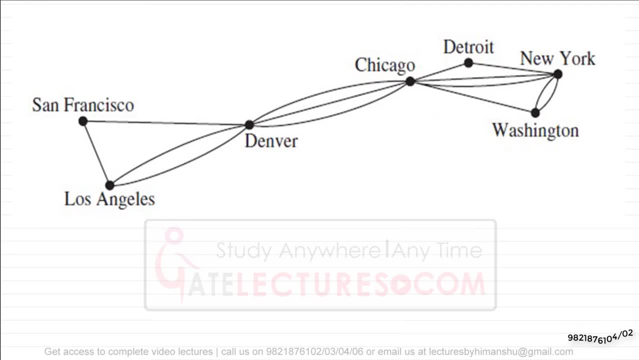 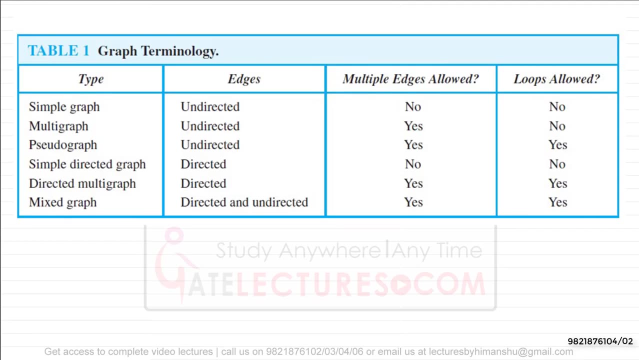 in in a multi graph, you say: uh, there are multiple edges allowed, but loops are not allowed. okay, so this is clearly. clearly, we are saying it is a multi graph because multiple edges are allowed are not allowed. now, if you see this example, this example is representing a pseudograph, pseudograph. 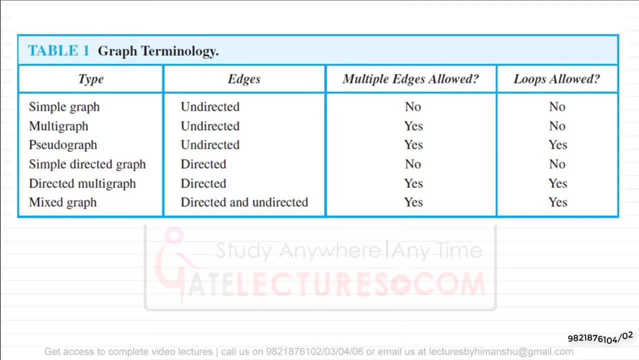 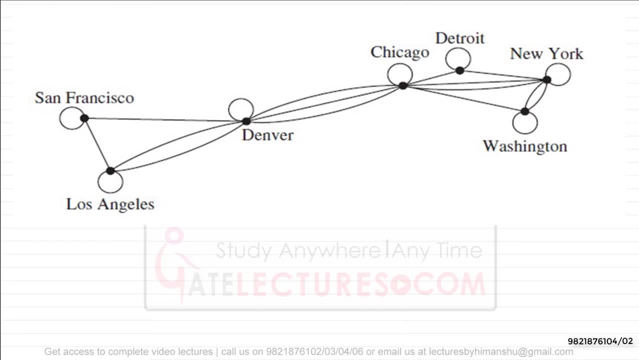 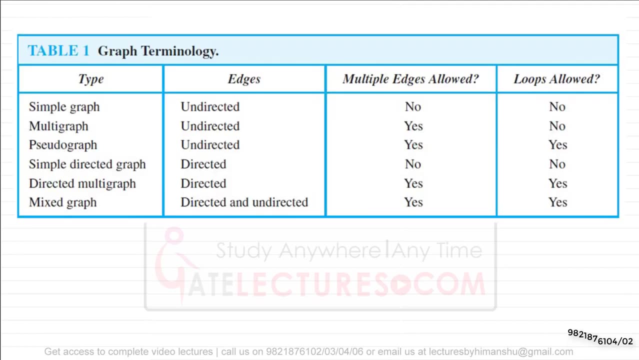 means the graph is undirected. multiple edges are allowed as well as loops are allowed. so because between every city here the loops are also allowed and multiple edges are also allowed. so this is a pseudograph. then we have this graph which is representing, uh, the simple directed graph. 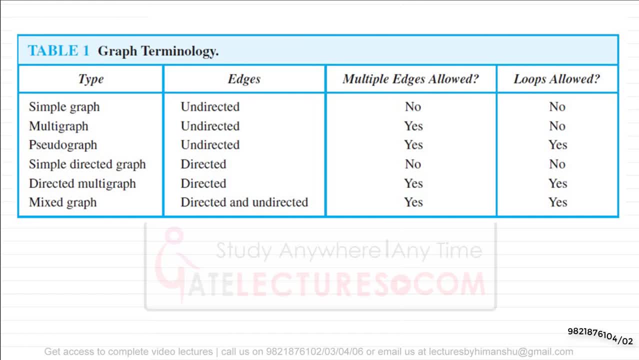 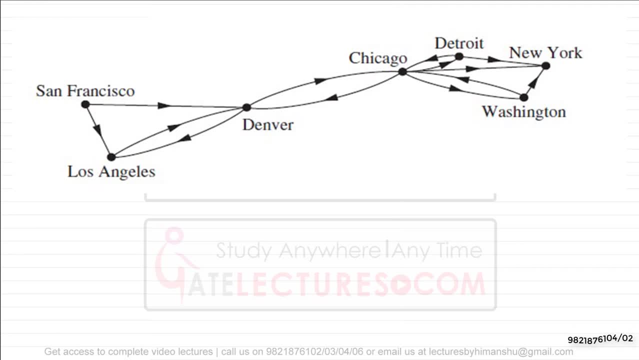 that means multiple edges are not allowed, loops are not allowed, but directions are allowed, so you can have. you can see, between every pair of cities here there are given some directions, like, for example, between san francisco and denver. we have a direction and that means we have an edge between san francisco to denver. 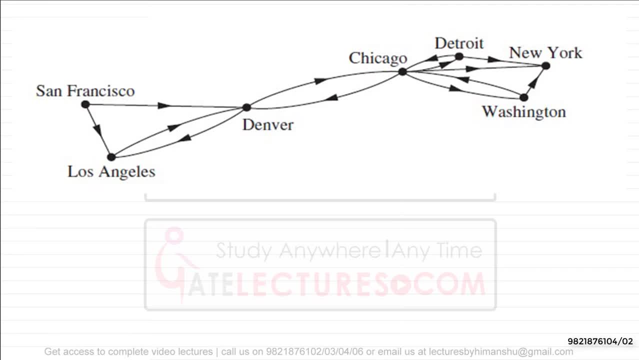 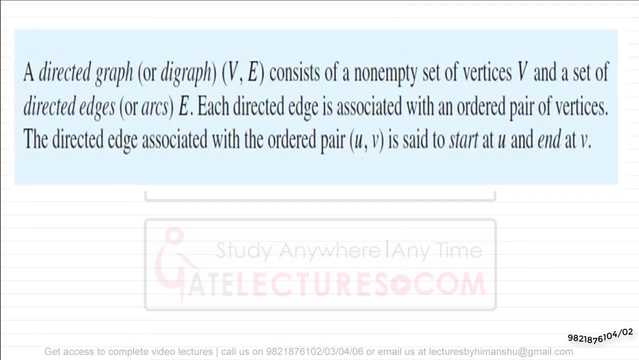 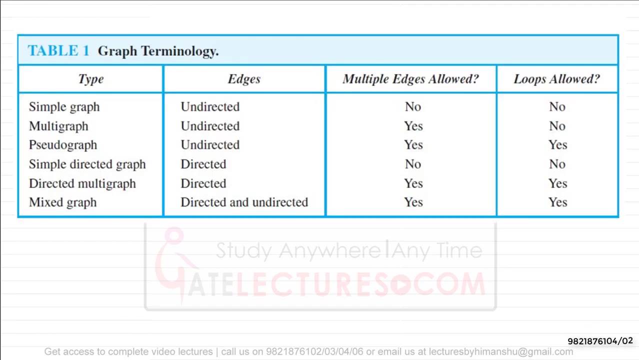 but we do not have any edge between denver to san francisco. then we have los angeles and so on. okay, because their directions are given for this graph. now, this graph was simply representing a simple directed graph. in the same way, we can have directed multigraph and we can. we can have 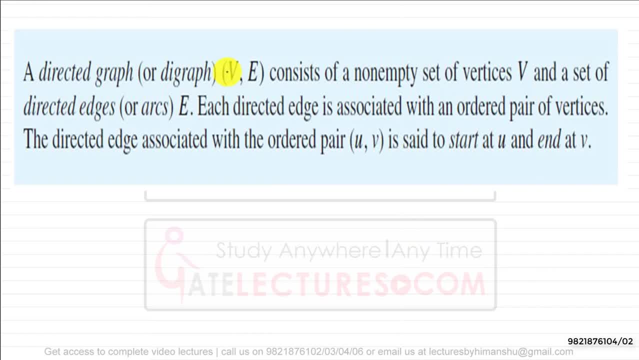 mixed graphs. now look at the definitions here. what is a directed graph? a directed graph or diagraph is represented by v comma e- there is set of vertices, and e is a set of edges, which is consisting of a non-empty set of vertices. see wherever we are discussing. 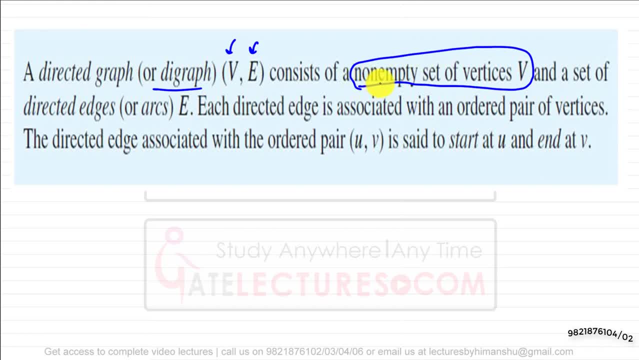 about graph definition. it is always non-empty set of vertices, because without having any vertex a graph cannot exist, and a set of directed edges you see in, without the having having an edge, a graph can exist. for example, if i say we have three vertex- v1, v2 and v3- now even if there is no edge between these, 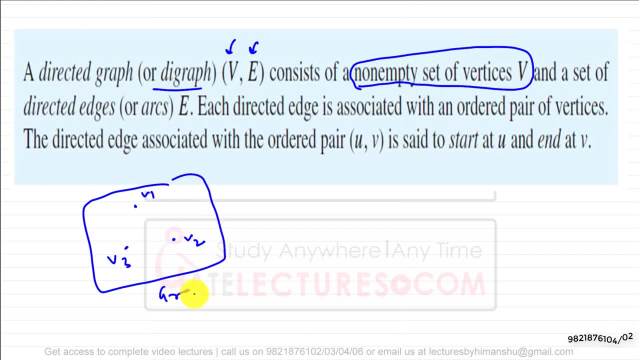 three vertices, but still it is called as a graph. okay, so for a graph, having a vertex is important, or you can say it is mandatory or it is necessary, but having an edge it is not at all necessary. now, each directed edge is associated with an ordered pair of vertices and the directed edge 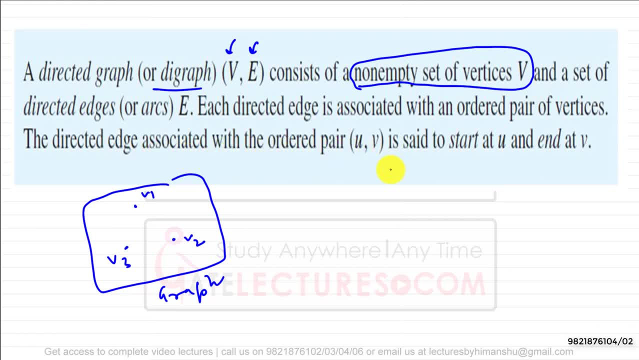 associated with the ordered pair is said to start from u to endpoint of v. so this is just a definition of directed graph. what does it mean? it is saying that if we have three vertices- v1, there is a vertex v2 and there is a vertex v3, now a directed graph v, comma e consists of non-empty. 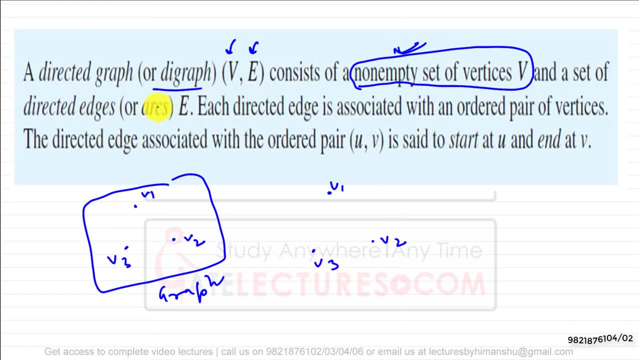 set of vertices. yes, it is a non-empty set of vertices and set of directed edges, like, for example, between v1 to v2. there can be an edge. there can be an edge between v1 to v2, right. in the same way, we can have an edge between v2 to v3. we can have an edge between v1 to v3, okay. 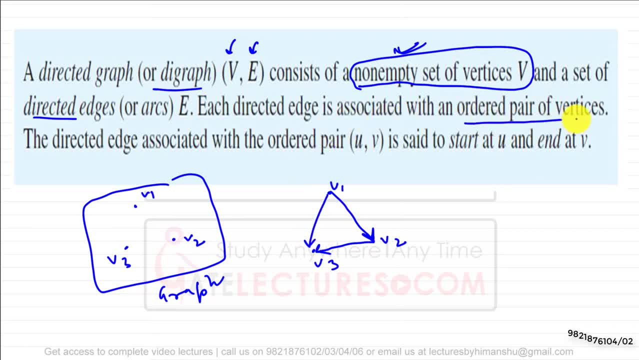 so each directed edge is associated with the ordered pair of vertices. ordered pair of vertices mean that means between v1 to v2 we can have an edge, but between v2 to v1 we do not have an edge. okay, so v1 comma v2, this ordered pair is not at all equivalent to v2 comma v1. So these two ordered pairs are not at. 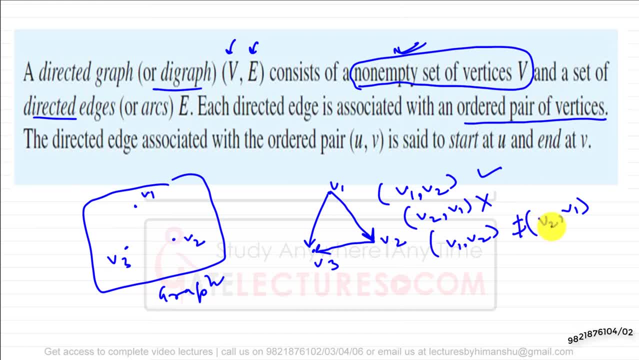 all equal. So that is why we say, when we represent the set of edges, then it should be an ordered pair. Now, what does it mean when I am saying ordered pair? Assuming this is one graph: this is vertex v1,, this is vertex v2 and this is vertex v3. Now, this graph is a completely 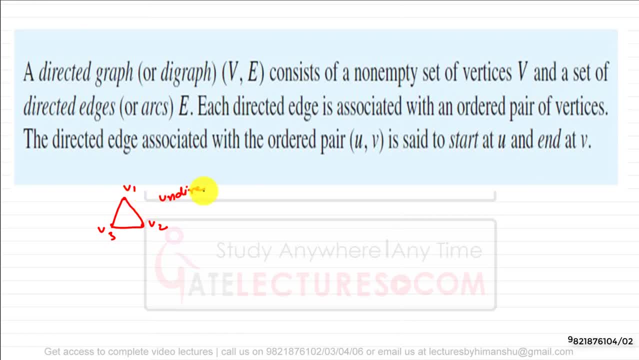 undirected graph. This is a undirected graph. Now, if I am showing what are the vertices we have, or what are the edges we have, then we can have three kinds of representations. Number one: we can have adjacency list representation. Second one: we can have adjacency matrix. 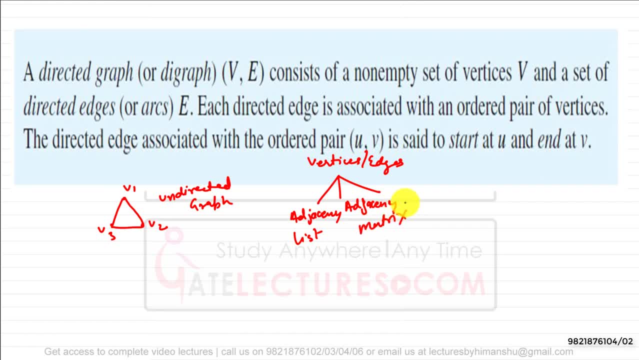 representation. And third one is: we can have set representation. Now we have already seen the adjacency list and adjacency matrix, representation in data structures also, And in the coming videos we are also going to discuss about the adjacency list as well as the adjacency matrix. But here we are represent. 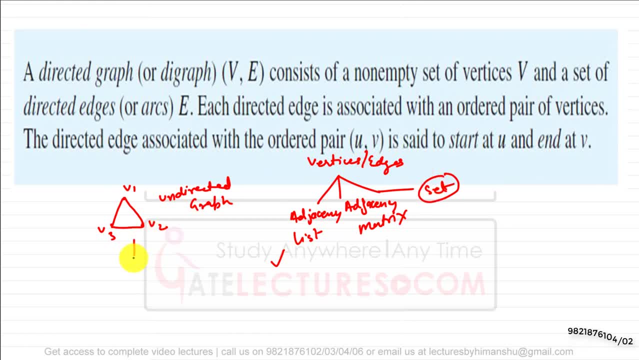 using the set representation Now, when we have undirected graph. now here we have in this set we represent unordered pair of vertices. unordered That means we can have v1 comma v2,. there is an edge Between v2 comma v3,. there is an edge Between v1 comma v3,. there can be an. 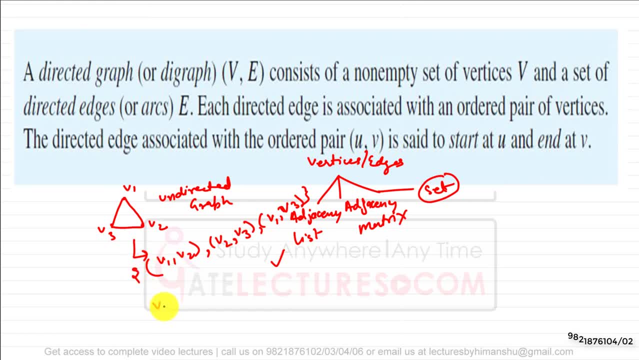 edge. It represents that v1 comma v2 is equivalent to saying v2 comma v1.. This is in case of undirected graph. That means the order does not matter. v1 comes first with v2, that does not matter. But when we have a directed graph, directed. 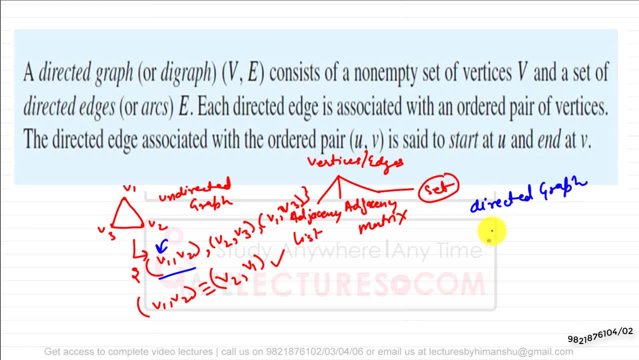 graph. Directed graph means we can have vertex v1,, v2, v3.. Now, in these three vertices, there is an edge between v1 to v2,, there is an edge between v2 to v3, and there is an 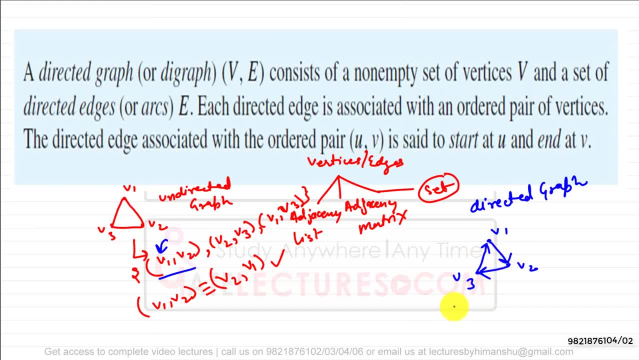 edge between v3 to v1.. Now how we are going to write the pair of vertices, pair of edges. We can have v1 comma v2.. We can have v2 comma v3.. We can have v3 comma v1. But we can have. 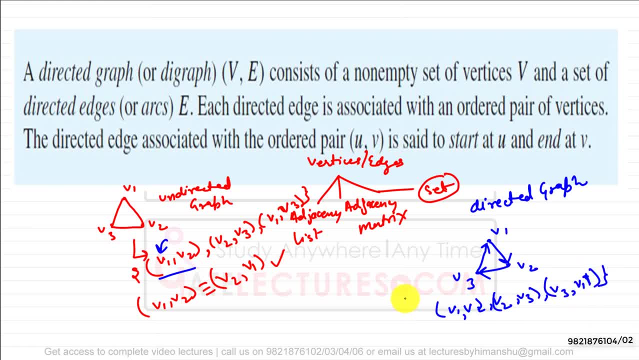 v2 comma v3. But we can have v2 comma v3. But it does not mean that v1 comma v2 is equivalent to v2 comma v1. Because when I am saying v2 comma v1, that means there is a directed edge between v2 to v1. So in case, 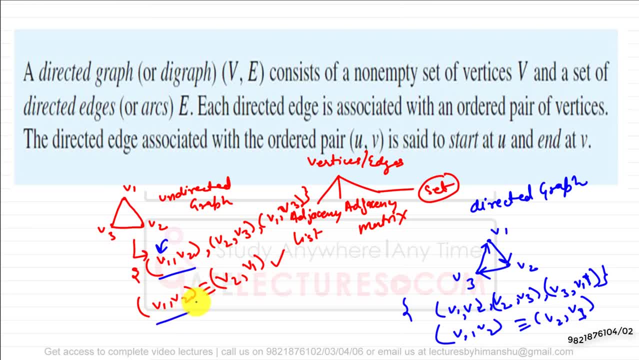 of undirected graph, we use unordered pair of vertices to represent an edge. But in case of directed graph, we always use ordered pair of vertices to represent an edge. Okay, So each directed graph is associated with ordered pair of vertices And a directed. 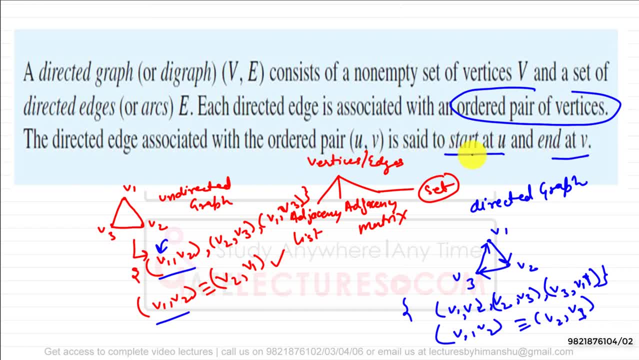 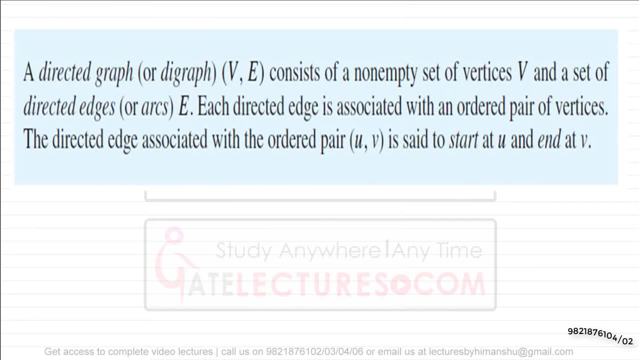 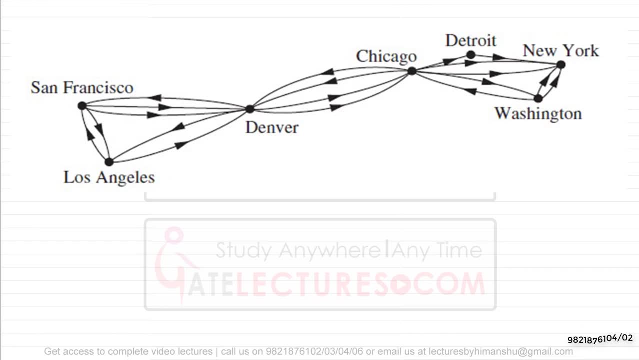 graph is associated with the ordered pair of vertices to start from u and end at v. For example, if I say u comma v, that means the edge is from u to v. Okay, Now here you can see all the edges that are represented in this graph. they are: 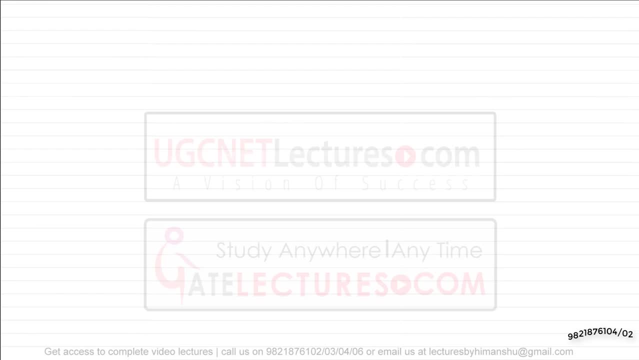 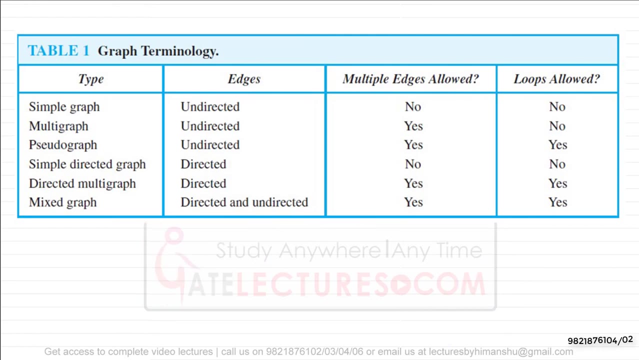 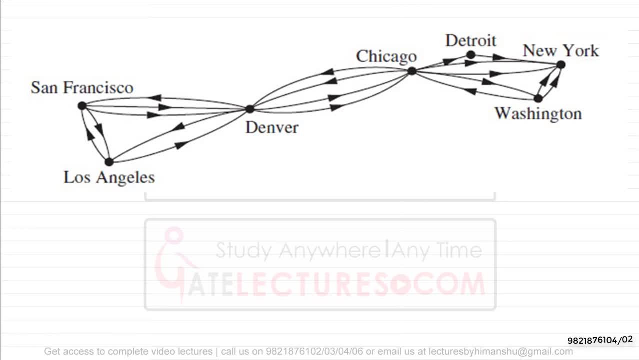 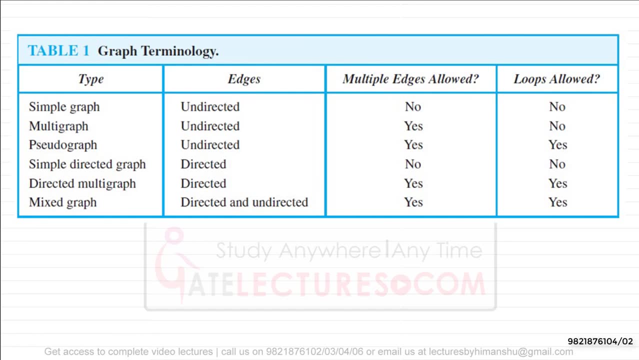 where we were having all the directed edges. we do not have any loop in this graph, so this graph is representing a directed multi-graph. directed multi-graph: okay, there are multiple edges are allowed as well as loops are allowed, but it is not representing a simple graph. why it is not? 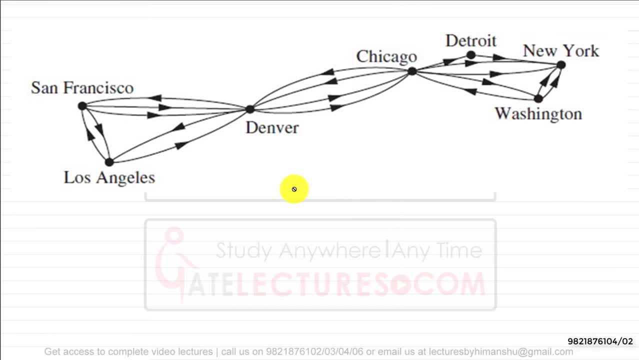 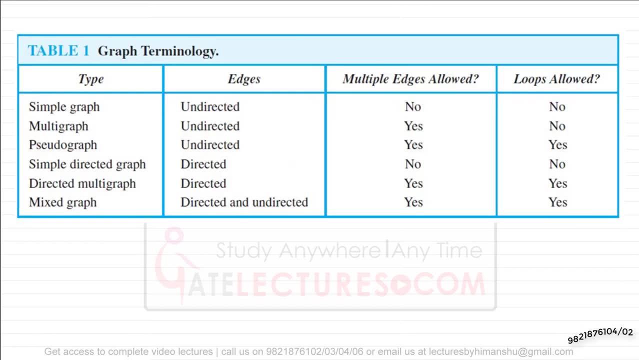 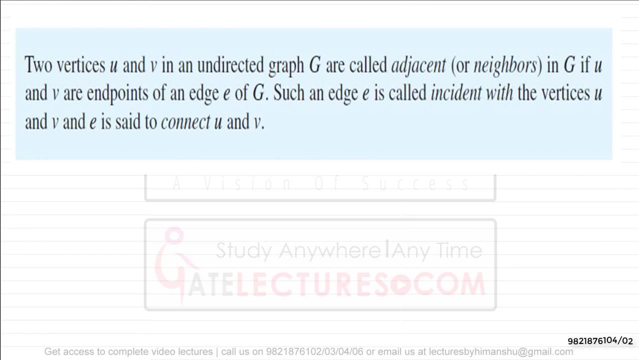 representing a simple graph, because if you see that between san francisco and denver, there are two paths are possible, there are two, two edges with the same directions are possible. therefore, it is representing a directed multi-graph, correct? now look at this. this definition is saying two. 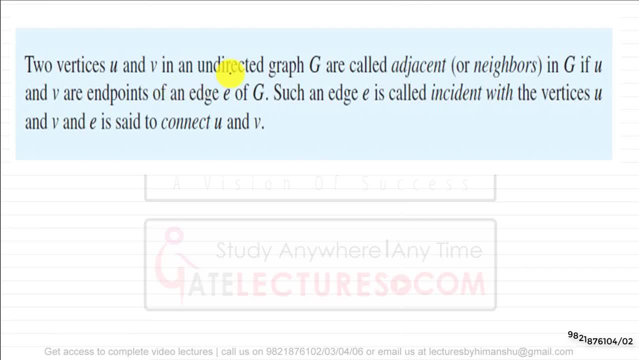 vertices u and v in an undirected graph, g is called adjacent. if in g, if u and v are endpoints of an h of g, h, e of g, such that e is called incident with the vertex u and v and e is said to connect u you. 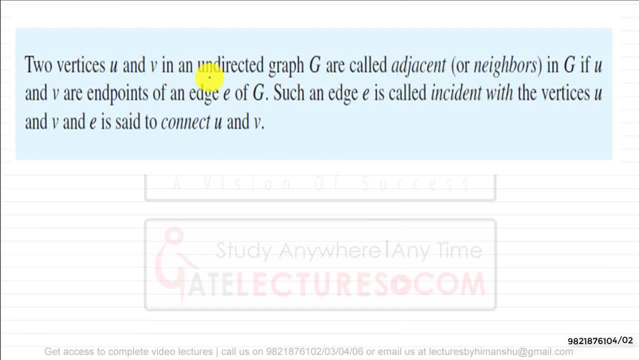 you and v. that that means, first of all, they are discussing about the undirected graphs, where no directions are given. now, if there is a vertex u and there is a vertex v, now these two vertices are called as adjacent. adjacent when, and only when, there is an h which is existing between 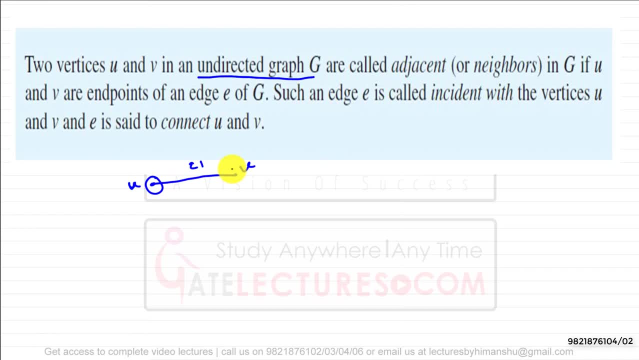 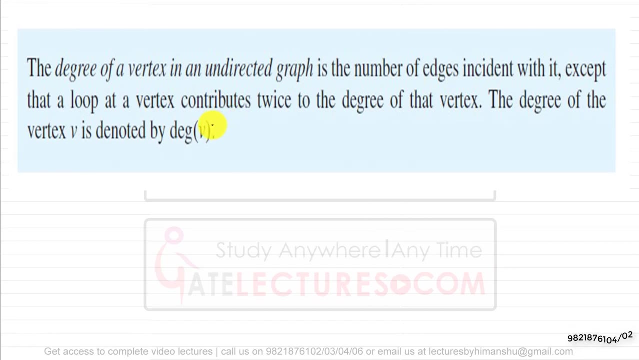 u and v, which is having one end point as u and second end point as v. okay, so such kind of uh vertices are called as adjacent vertices. now look at this definition. a degree of a vertex in an undirected graph is the number of edges incident with it, except that a loop at a vertex 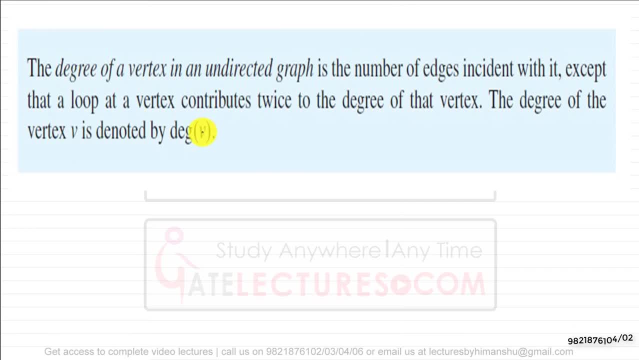 contribute twice to the degree of vertex. the degree of vertex v is denoted by degree of v. okay, what does it mean? it means, let us suppose we have, uh, these two different kinds of graphs. this is a undirected graph. this is v 1. vertex v 2: this is vertex v3. now, this is a second. 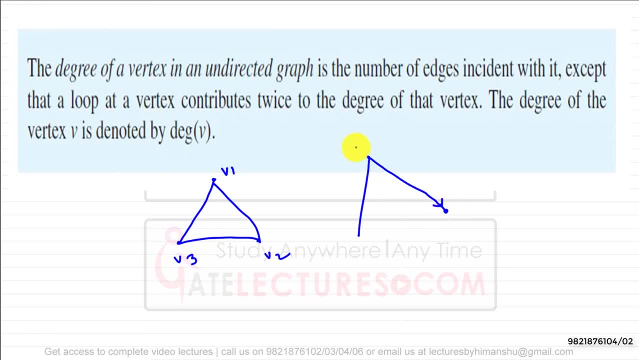 graph, which is a directed graph, directions are given. this is vertex v1, this is vertex v 2, and here it is vertex v 3, and this is presenting v 4, v 5 and y rightгр French chi, expect that an edge? okay, and we have one more graph here. this is vertex v1. this is vertex v2. there's a self loop. 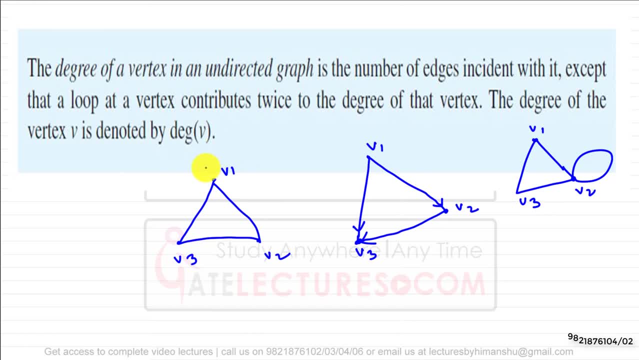 and this is vertex v3. now, when i'm saying a degree of a vertex in an undirected graph is the number of edges, incident with it. now, this is discussing about the undirected graph and they're saying the number of edges incident with it, incident with it, okay. now, for example, 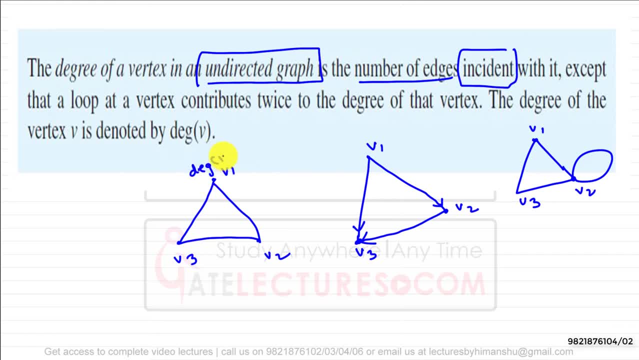 if i say what is the degree of vertex v1? degree of vertex v1 is what are the number of edges incident the vertex v1, which are 2. now, what is the degree of vertex v2? degree of vertex v2 that is equivalent to 2. what is the degree of vertex v3 that is also equivalent to 2? this is undirected. 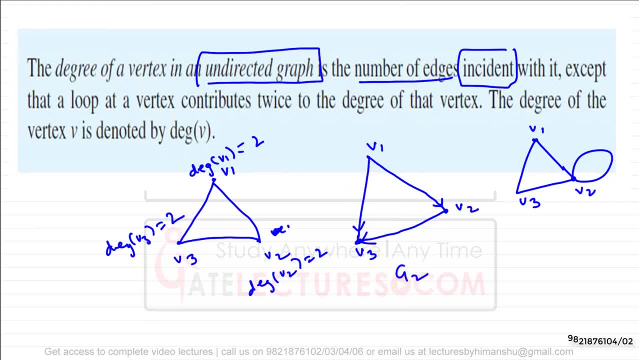 graph. now, second graph, this graph- g2 it is- is an undirected graph. now, if i say what is the degree of vertex v1? now, here, the degree of vertex v1 is zero because there is no incident vertex right now for a, for a directed graph, we'll 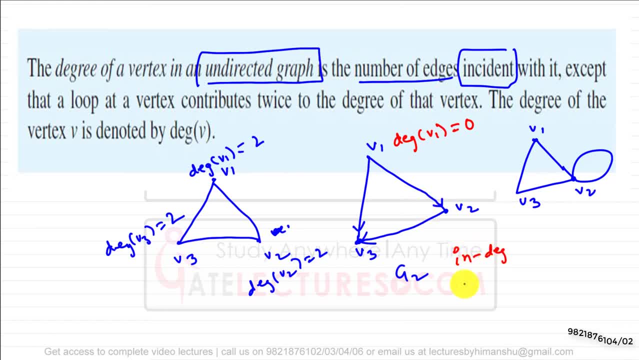 be discussing what? what is a in degree and what is a out degree? now, here we are just discussing about the out degree. now, what is the degree of vertex v2? degree of vertex v2 is one, because there's one incident in edge here- and what is the degree of vertex v3? that is equivalent to. 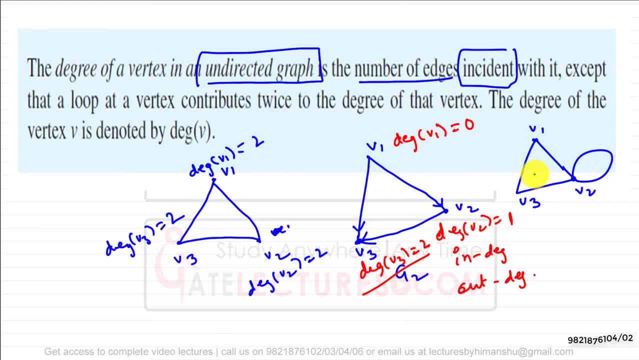 two in the directed graph. now the third graph, which is represented by this graph g3. now, this is undirected graph. what is the degree of vertex v1? degree of vertex v1 is 2, because there are two edges incident. what is the degree of vertex v2? vertex v2 degree is 1, 2, 3 and 4, so the degree of 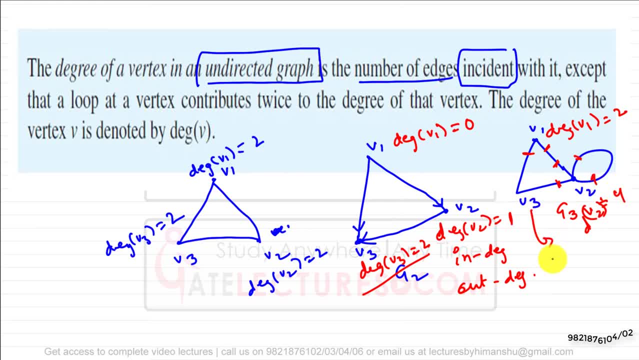 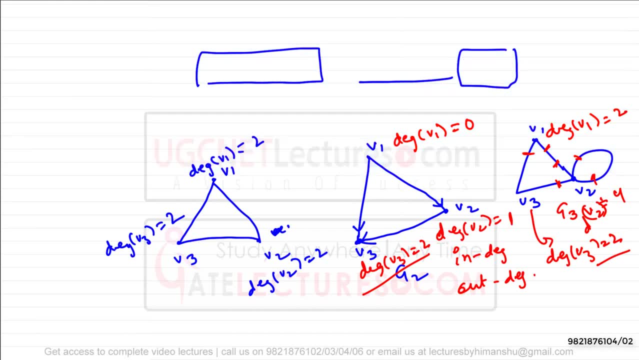 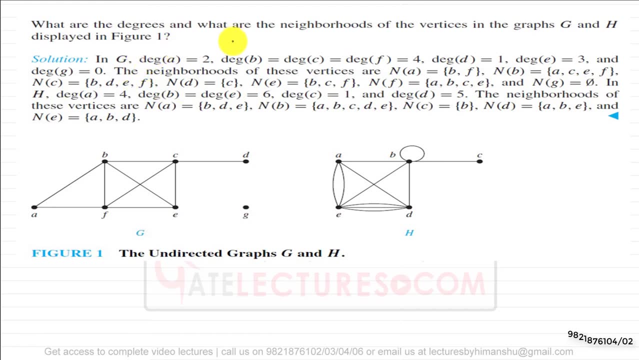 vertex v2 is 4.. in the same way, what is the degree? what is the degree of vertex v3? that is represented by two? so this is called as a degree of a vertex. Now look at this one, This question: what are the degrees and what are the neighbourhoods? 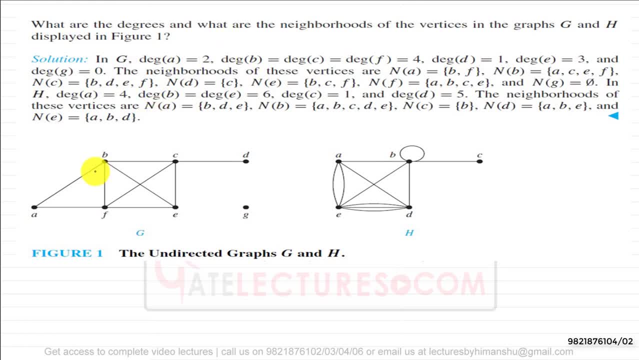 of the vertices in the graph G and B. Now you say: what is the degree of A? Degree of A is 2, because there are two edges. What is the degree of B? Degree of B is 1,, 2,, 3 and 4.. There are. 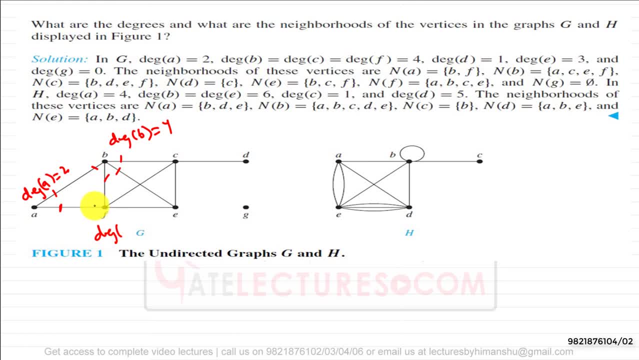 four edges. What is the degree of F? Degree of F is 1,, 2,, 3,, 4.. So there are four edges. What is the degree of vertex E, That is 3.. Degree of vertex C, That is 3. and degree of vertex D, That. 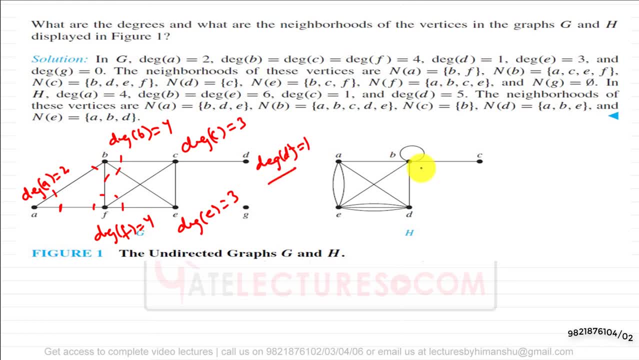 is equivalent to 1.. So there is a degree of each and every vertex here. Now look at this one here. What is the degree of vertex A? Degree of vertex A because there are multiple edges between two pairs of vertices. So here, 1, 2,, 3 and 4.. Now in this graph, because it is having multiple edges between the same. 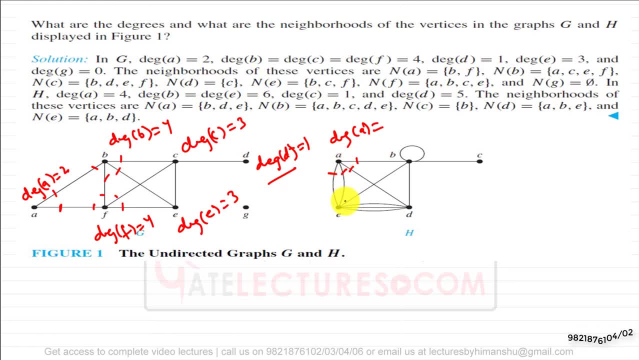 pair of vertices, like for example between A and E, there are multiple edges. Now, here the degree of vertex A will increase and degree of vertex A now will become 4.. But in the original case the degree of vertex A was only 2.. Now, what is the degree of vertex E? How many edges are there? 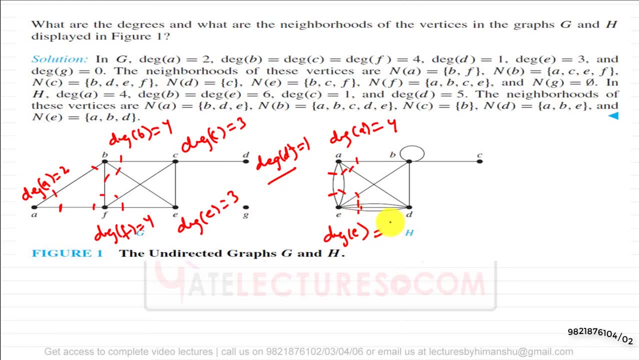 1,, 2,, 3,, 4,, 5 and 6.. So degree of vertex A is 6.. What is the degree of vertex B? Vertex B is 1,, 2,, 3,, 4,, 5 and 6.. 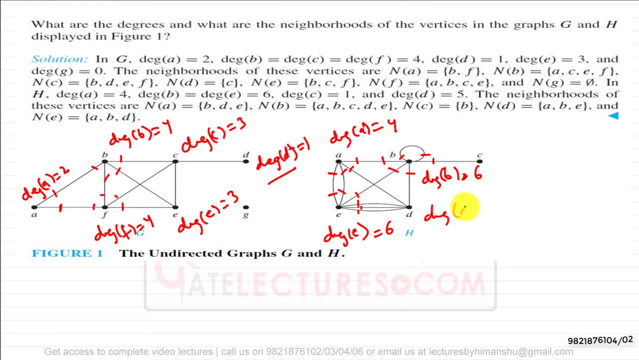 There are 6 degrees. What is the degree of vertex D? Degree of vertex D is 1,, 2,, 3,, 4, 5.. And what is the degree of vertex C? That is equivalent to 1 only. So this is representing a graph and we found out. 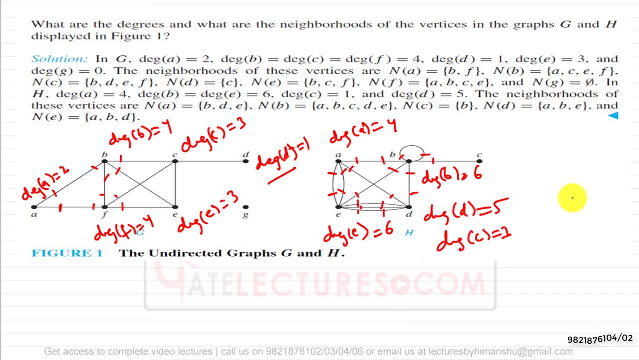 what is the degree of each and every vertex? Now, when I say neighborhood of every vertex, neighborhood, for example, here, for this particular graph, what is the neighborhood vertices of any particular vertex? For example, if I say what is the neighborhood of vertex A Neighborhood, are the vertices which are adjacent to A? B is adjacent? 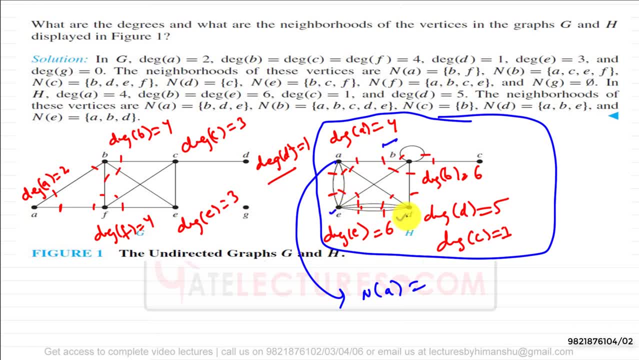 to A, E is adjacent to A and D is adjacent to A. So neighborhood of vertex A is B, D and E In the neighborhood of vertex B. So see, even if the degree of vertex B is 6, but the neighborhood can. 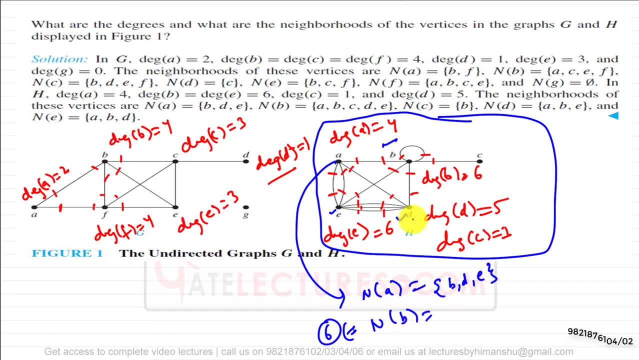 be less because vertex B is having self-loop. But still, what is the neighborhood of vertex B? That is A, B, C, D and E. So in neighborhood of B there are 5 vertices. 5 vertices but the degree. 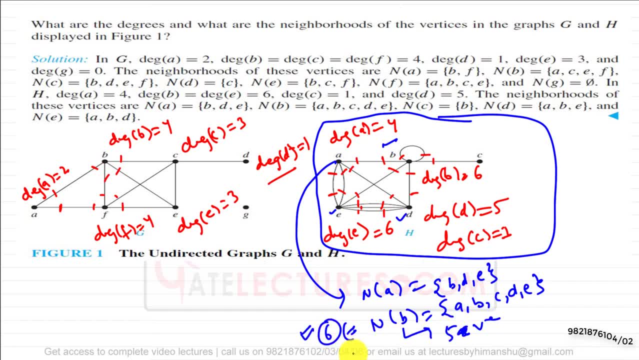 is 6.. That means if the degree is more than the neighborhoods, so they may. it may contain some kind of self-loop Correct. In the same way, if I say what is the neighborhood of D? So neighborhood of D is A, B, E. So in D we have A, B, E, Correct, But still there's 3 vertices. 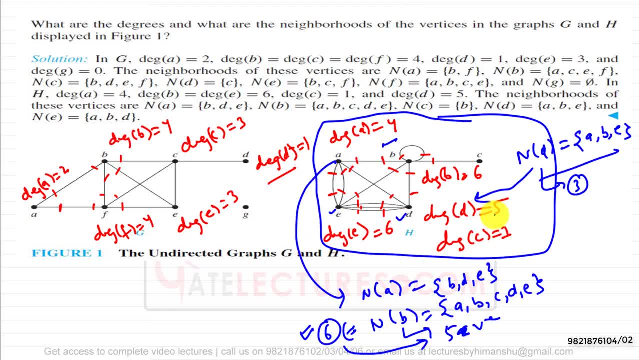 in the neighborhood but the degree of D is 5.. So still, because there's a degree of D is 5 and neighborhood of E, it is having 3.. So either D can be having any kind of self-loop or